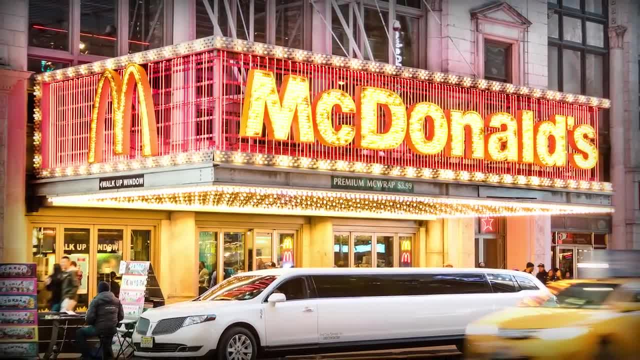 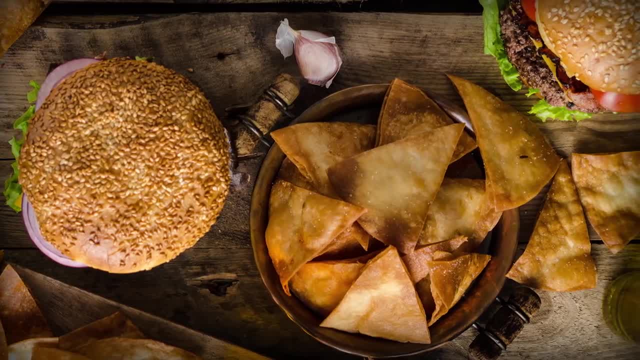 then everyone will just go to their competitor, And if McDonald's and Burger King both try to raise their prices at the same time, some other company will enter the market, since the barriers are relatively low. Taco Bell will start selling hamburguesas. The last type are oligopolies, and that's what we're going to focus on today. 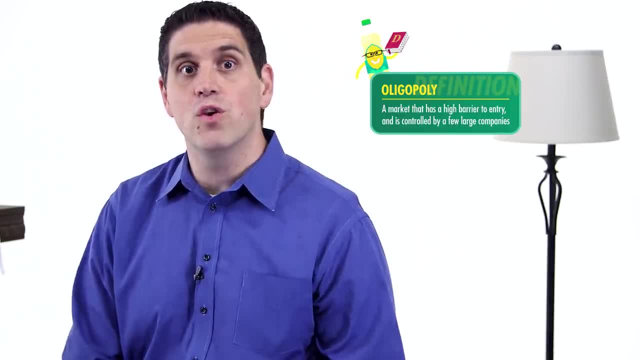 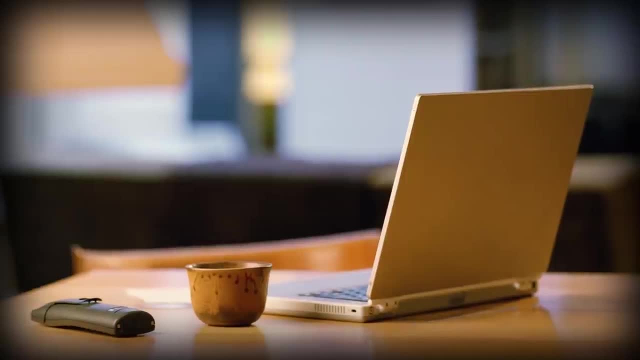 Oligopolies are markets that have high barriers to entry and are controlled by a few large companies. Oligopolies are all over the place. In fact, their products are likely in front of you right now. The laptop computer market is dominated by companies like HP. Dell and Apple, and the majority of mobile phones are produced by Apple, Samsung and LG. You also see this type of thing in the market for cars, air travel, movies, candy and game consoles. Like monopolistic competition, oligopolies often sell products that are similar. but not identical, and this gives them some control over their prices. But how much You might love your iPhone, but if Apple raised the price of a phone to $3,000, you might switch to Android, But the price of an iPhone is pretty close to the price of a. 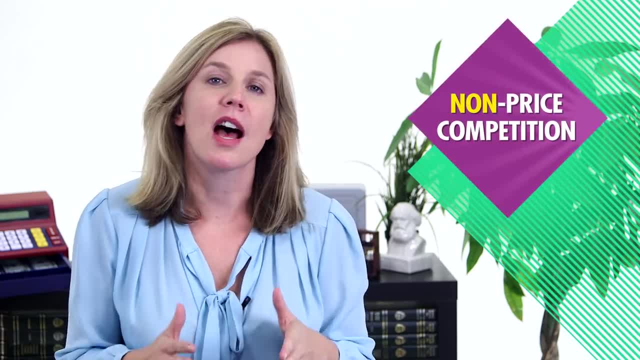 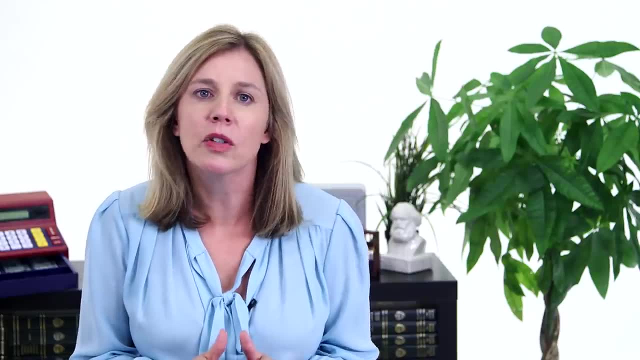 high-end Android. So how do they compete? The answer is non-price competition and, as you might guess, it's competing without changing the price. This happens in a lot of industries. Companies focus on things like style, quality, location or service. 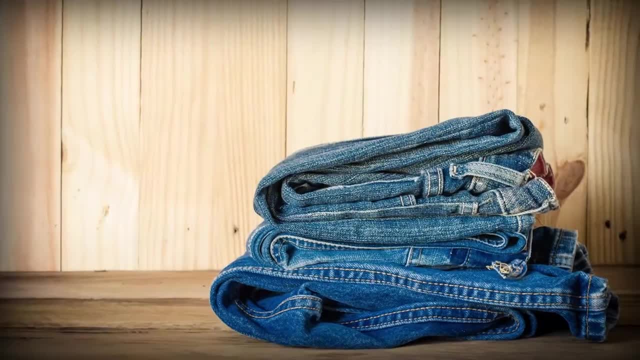 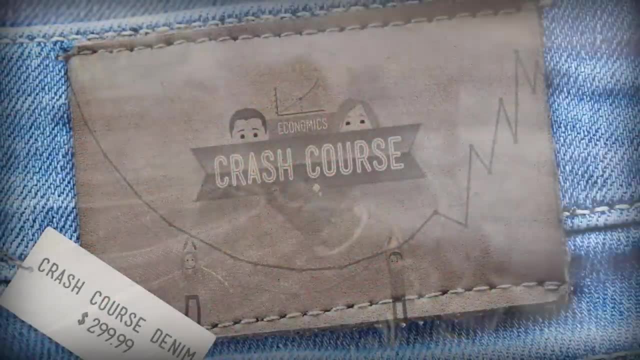 The goal is to distinguish their product from their competitors. Like the jeans that one company sells might be virtually identical to everyone else's in terms of quality, but if they can convince consumers that having a designer label on their butt is cool, buyers might pay much. 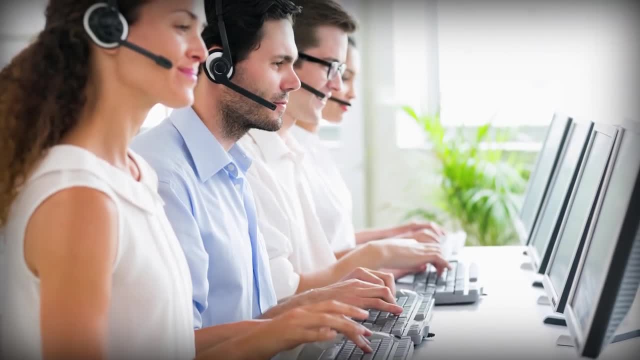 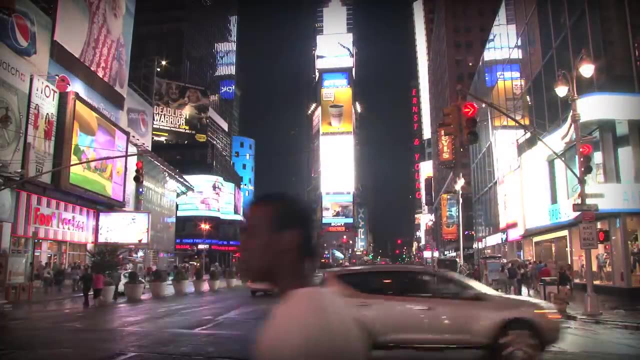 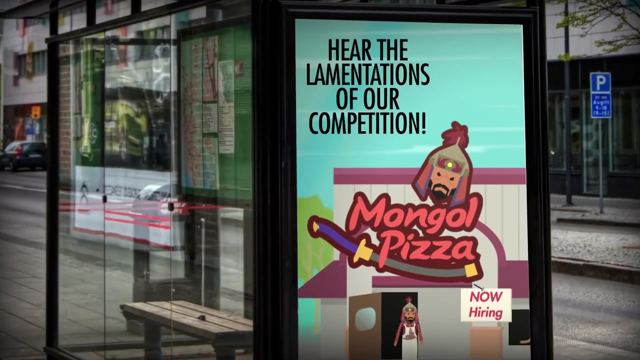 much more. The same logic holds true if a company has better customer service or has more convenient locations. The most recognizable form of non-price competition is advertising. Companies spend billions of dollars each year introducing new products or services and differentiating themselves from their competitors, And despite 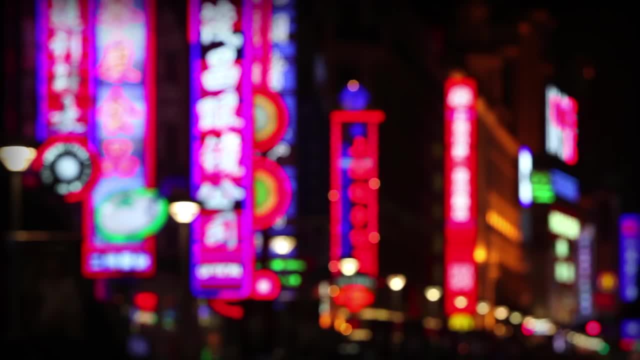 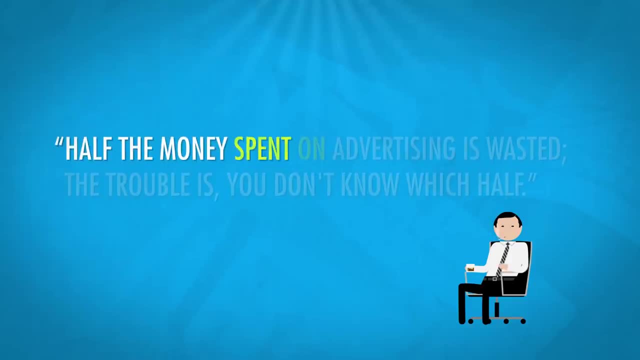 all that spending most of the time advertising just kind of fades into the background. Can you remember the ad that ran before this video? Nope me, neither Don Draper might tell you. half the money spent on advertising is wasted. The trouble is you don't. 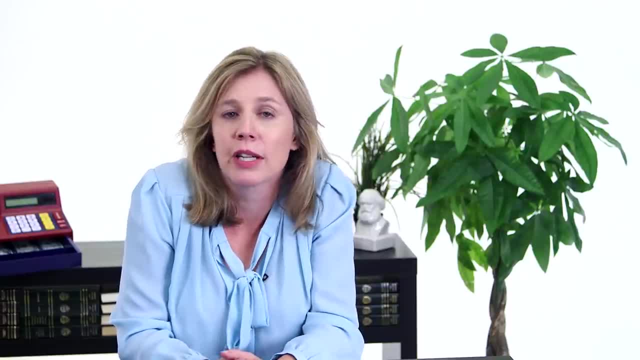 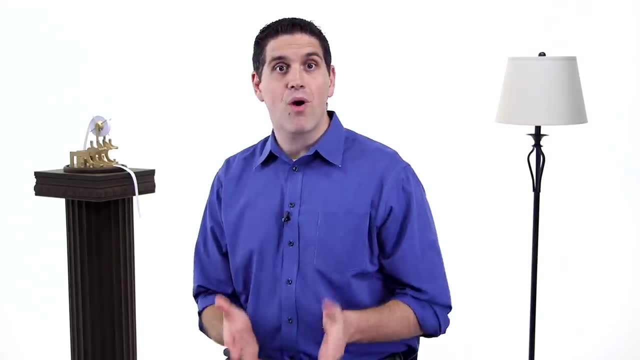 know which half. It's clear that not every advertisement sticks, but advertising can work to stand out. So those ads that run before YouTube videos Some of her products sold in monopolistically competitive markets, but the majority are probably from oligopolies. I mean think of 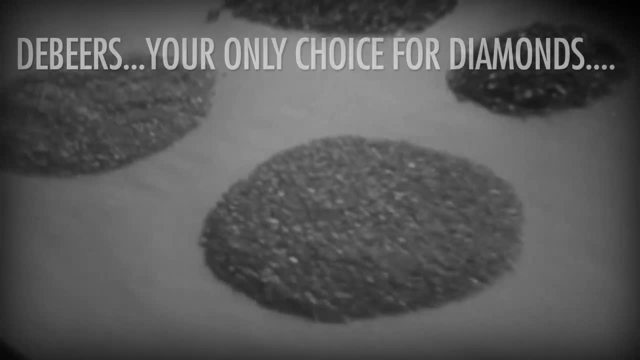 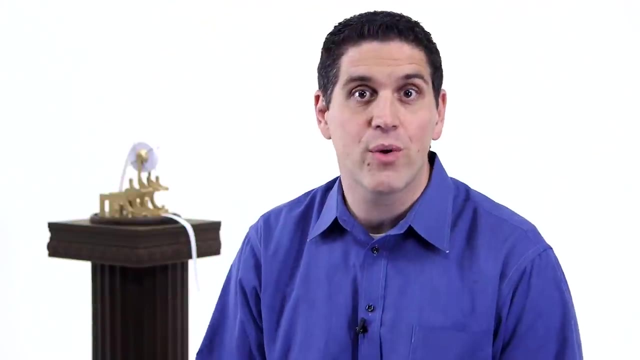 car companies, They advertise a lot. Generally, monopolies don't bother advertising because they have no competition and firms in perfectly competitive markets don't run ads because their products are identical. Advertising just increases their costs and drives up the prices, which means customers go to their competitors. So oligopolies sound like they operate pretty much like monopolistic competition. but the big difference between the two is that oligopolies are made up of a few large companies. So let's say you're a car company and you're selling a car. and you're selling a car and 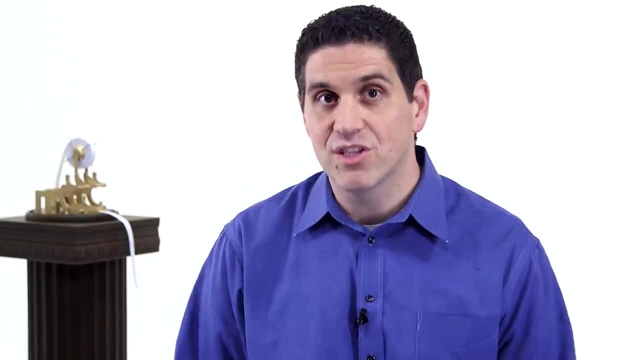 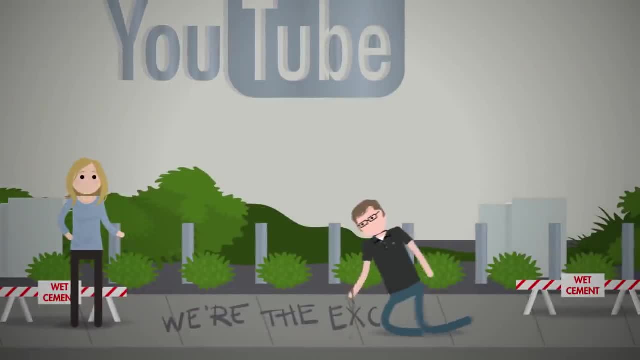 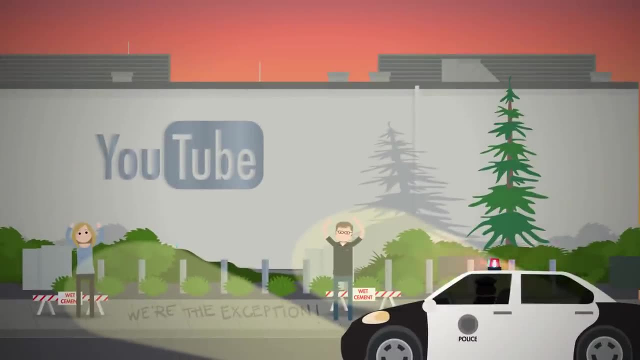 strategic decision-making. Let's go to the Thought Bubble. Let's start with a classic of game theory, something called the Prisoner's Dilemma. Suppose, Stan and I are arrested for scrawling in wet cement outside the YouTube studios. We're being interviewed separately. If we both confess, we'll both have to pay a $10,000 fine. 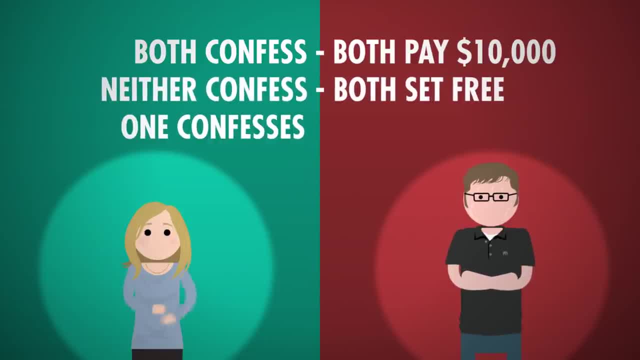 If neither of us confesses, we'll get off scot-free. And if I take a deal and confess but Stan doesn't, I'll walk away and Stan will owe $20,000, and vice versa. So what do we do? Because we can't discuss it. we both confess and both end up owing $10,000.. 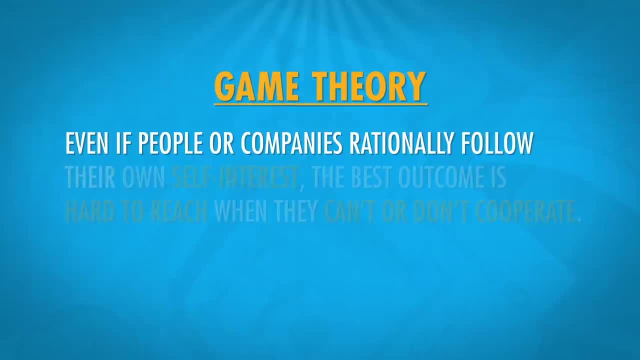 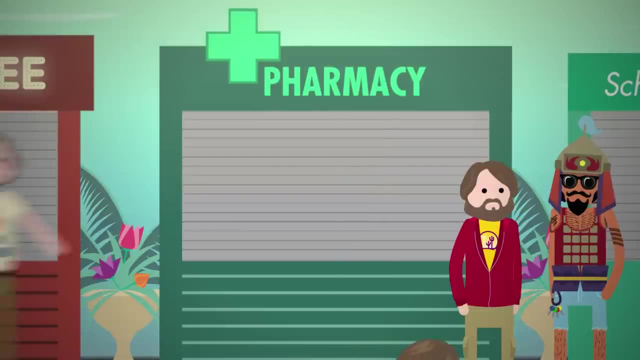 This is game theory. Even if people or companies rationally follow their own self-interest, the best outcome is hard to reach when they can't or don't cooperate. Game theory helps explain why you get drugstores and coffee shops right next to each other. 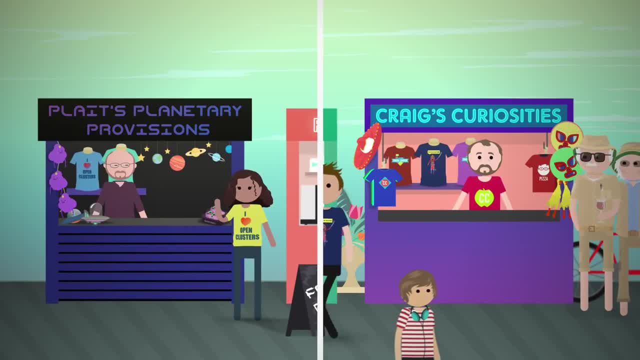 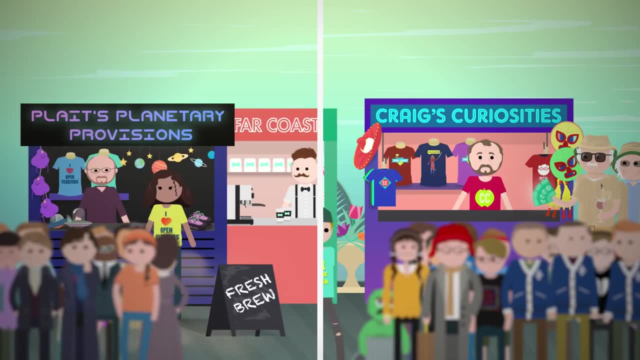 Let's say that Craig and Phil both start selling tchotchkes on the Coney Island boardwalk. At first they start on Optical, Then they go to the opposite sides of the strip sharing customers. equally, Phil realizes that if he gets closer to Craig he'll retain all of his old customers and snag some of Craig's. 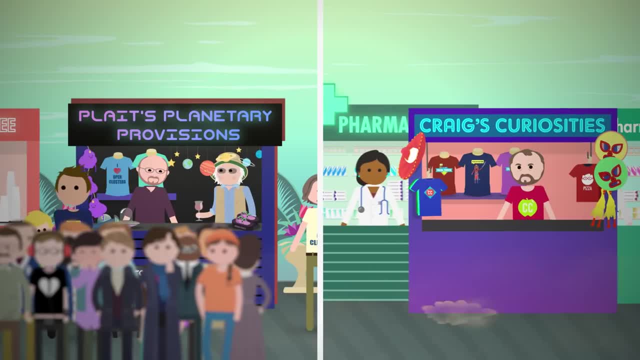 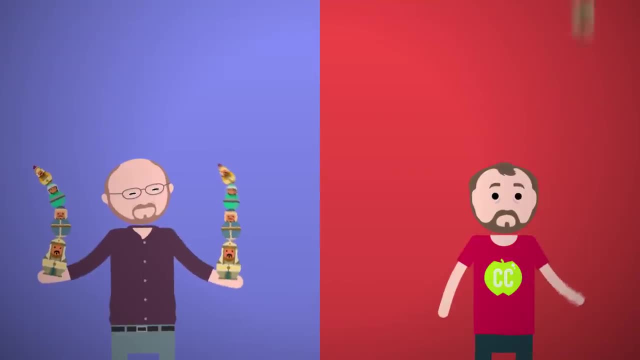 But Craig's no dummy. He moves his cart closer to Phil's. This continues until they both wind up right in the middle of the boardwalk, sharing customers equally and unable to improve their position. This also plays out with pricing, If Craig lowers his price on Crash Course nesting dolls. 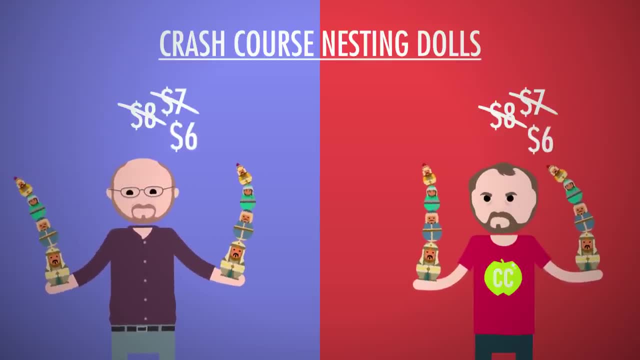 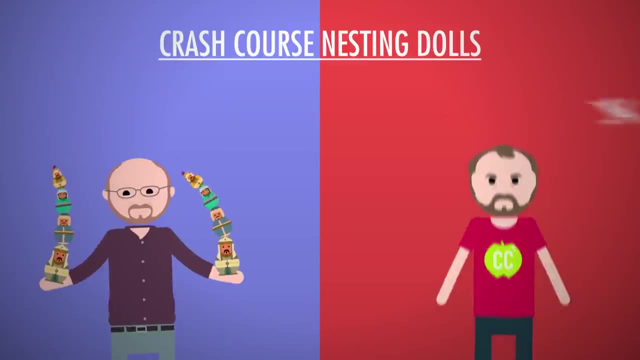 Phil will likely compete by dropping his prices as well. In the end, they're going to continue to share customers equally and earn less money. If Craig understands game theory, he knows there's no reason to change his price. Instead, he focuses on providing knick-knacks that differentiate his kiosk from Phil's. 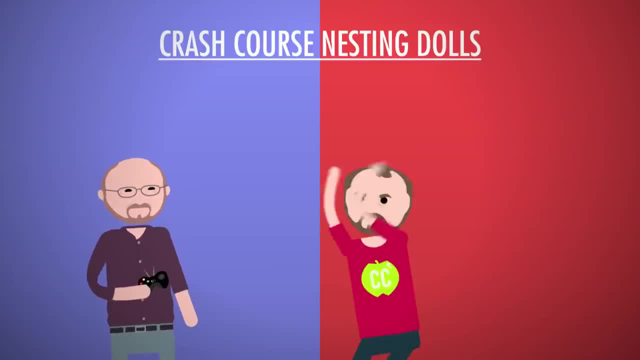 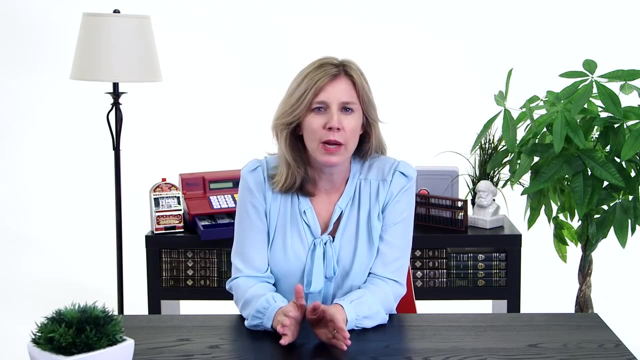 This can help explain why prices in oligopolies tend to get stuck and why companies focus so much on non-price competition. Thanks, Thought Bubble. So what if Craig and Phil don't compete at all? What if, instead, they agree to charge the same price? 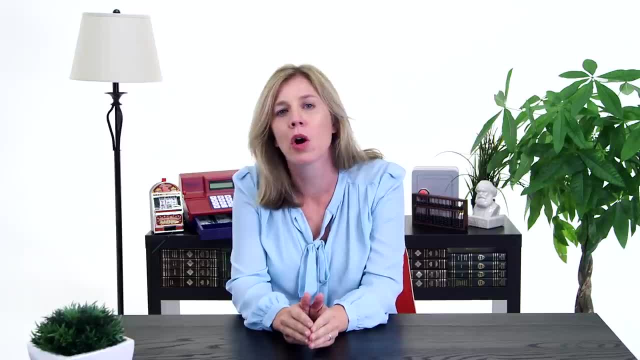 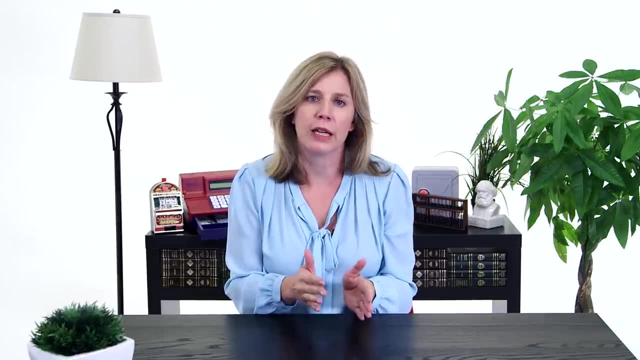 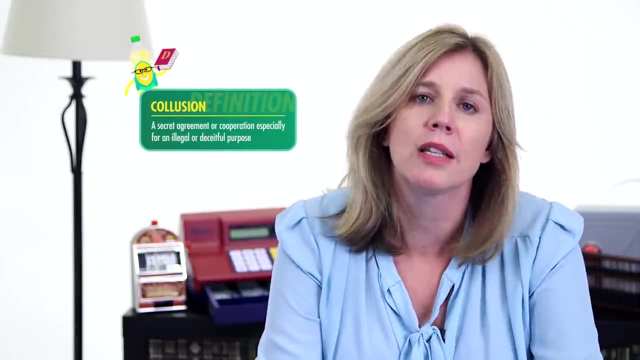 Conspiring to form what economists call a cartel. Again, they split the customers 50-50,, but now they make even more profit, benefiting at the expense of consumers. This is called collusion and it's illegal in the US. There are strict antitrust laws designed to prevent it. But that doesn't mean companies don't figure out other ways to raise prices. Price leadership is when one company changes its prices and its competitors have to decide if they're going to follow suit, Since they're not all the same. if they're actively colluding, it's technically legal. 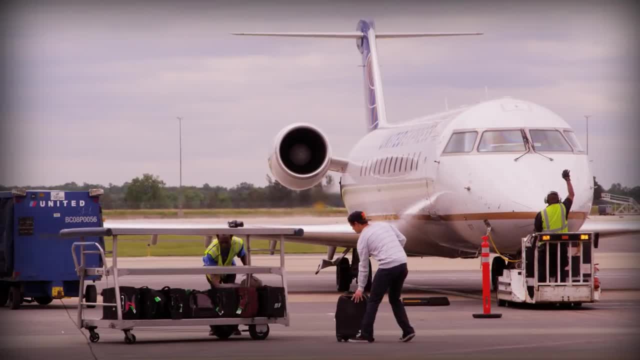 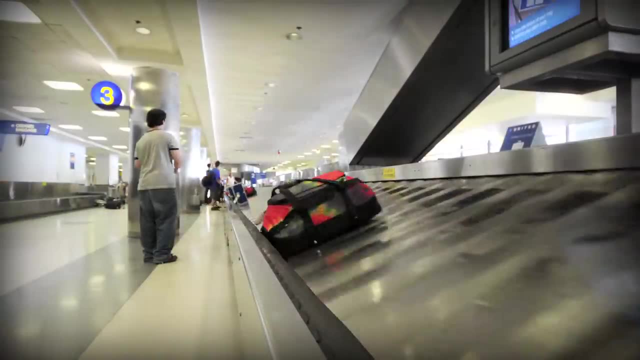 But it can be hard to tell the difference. Look at airline baggage fees. When some airlines started charging fees for check bags, other airlines quickly join them, And when one big airline changes their baggage fee, the others tend to move to the same price point. 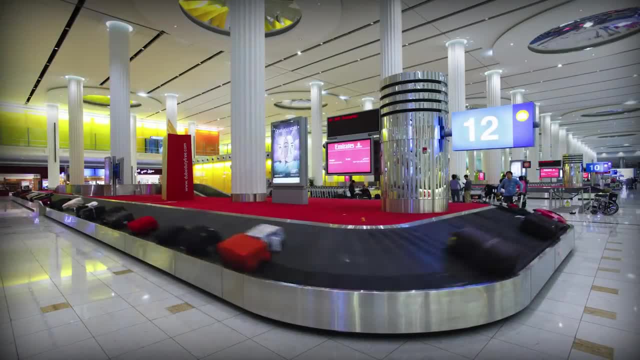 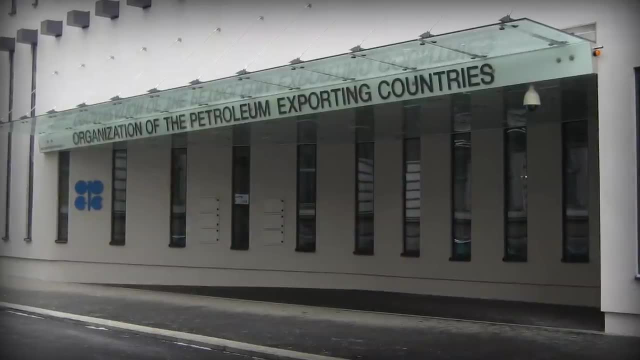 Are they colluding, Or is this a case of price leadership? Well, the Justice Department's looking into it. Other countries' laws differ and cartels do exist. The best example is OPEC, the Organization of Petroleum and Air Transport. 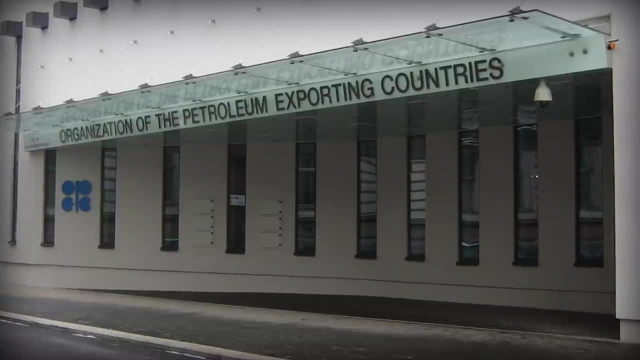 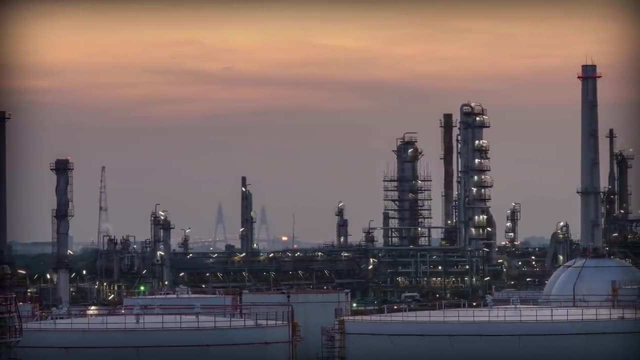 which controls the prices of petroleum-exporting countries. It's an international cartel made up of 12 oil-producing countries that manipulate oil supplies to control prices. They control 80% of the world's known oil reserves and nearly half the world's crude oil production. 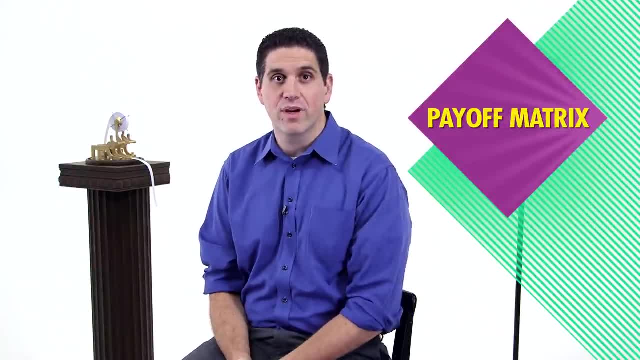 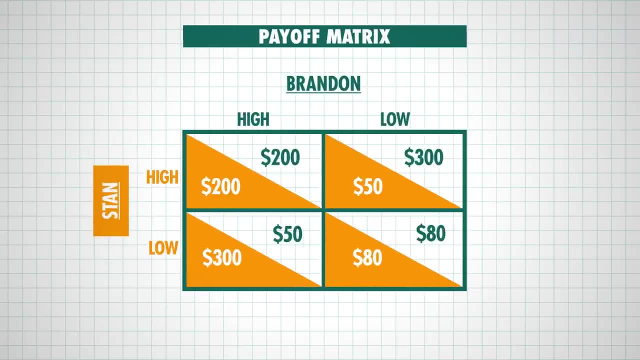 Economists like to explain oligopolies in game theory by creating something called a payoff matrix. Let's say Stan and Brandon have competing companies. Each can set prices high or low. The numbers in the boxes represent the amount of profit they can make in different situations. 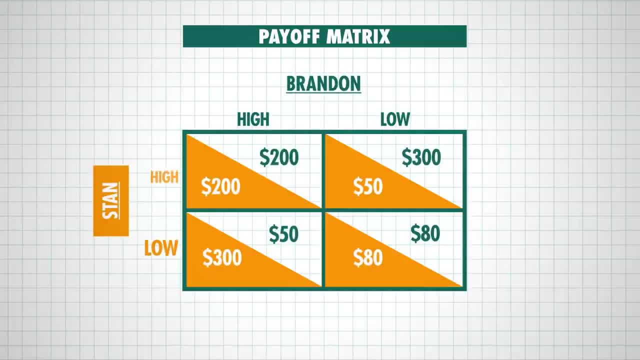 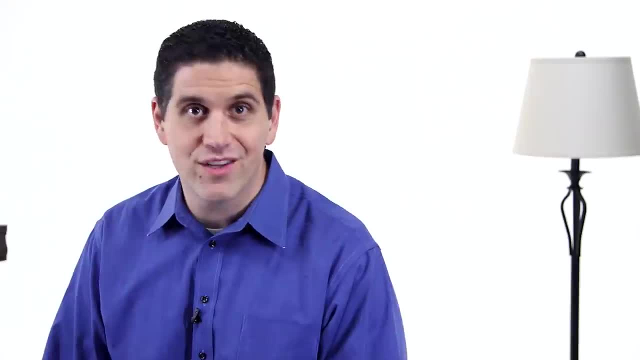 The profit on the left in each cell is for Stan and the numbers on the right are for Brandon. So if Stan has a low price and Brandon has a high price, Stan earns $300, and Brandon earns $50.. Now payoff scenarios for companies are never this transparent. 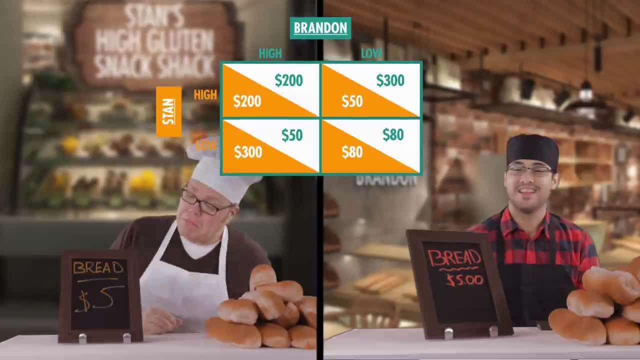 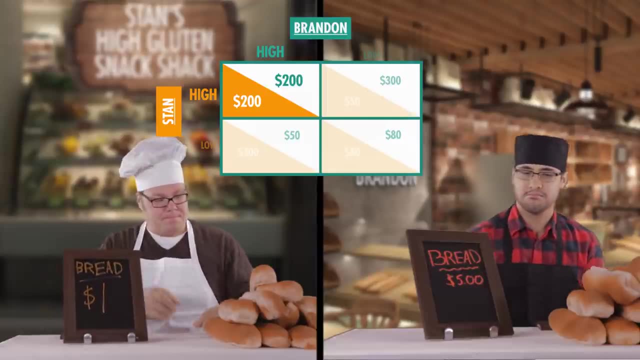 but the matrix says a lot about oligopolies. The optimal outcome is for each business to charge high prices, so they both get $200.. Stan knows this, but he also recognizes that there can be even more profit by charging a lower price. 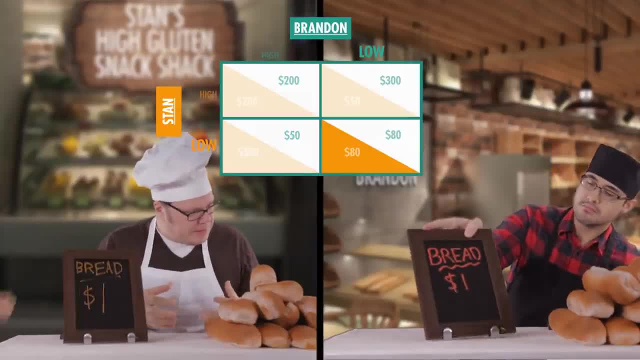 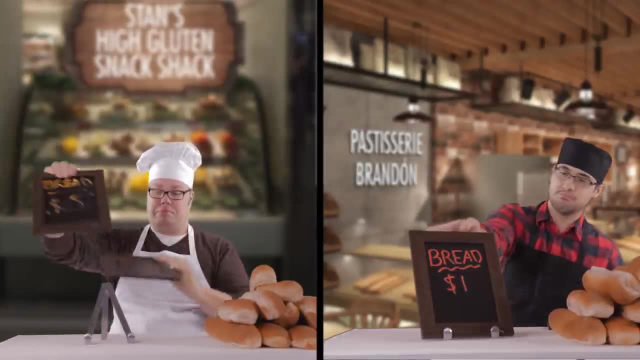 Brandon comes to the same conclusion. so they both price low and they end up getting $200.. They end up at the worst combined outcome, with each only making $80 profit. Even if they collude and agree to price high, they both have an incentive to cheat on that agreement. 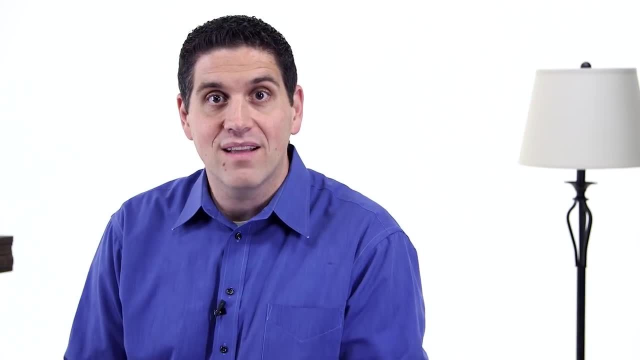 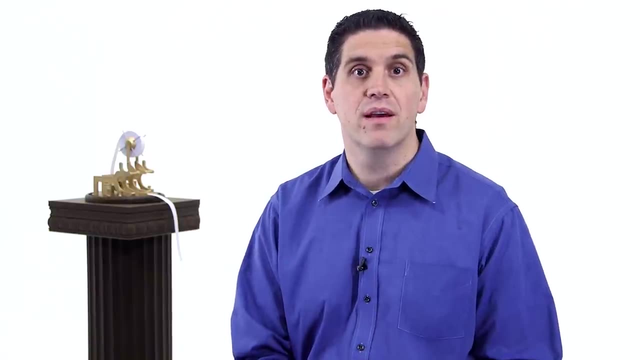 So collusion and cartels are often unstable. They can only last if the agreement is monitored and strictly enforced. A lot of times it's possible to predict the final outcome based on the information in the payoff matrix. The best outcome for Stan when Brandon makes a move.